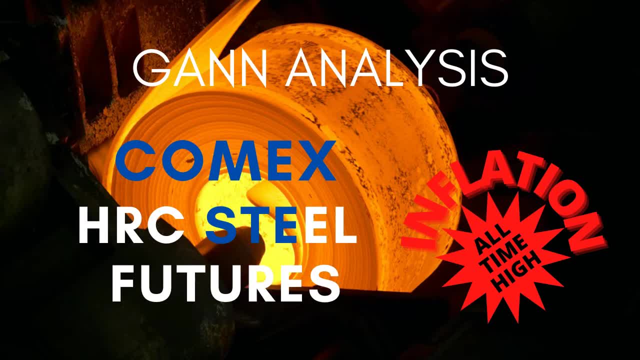 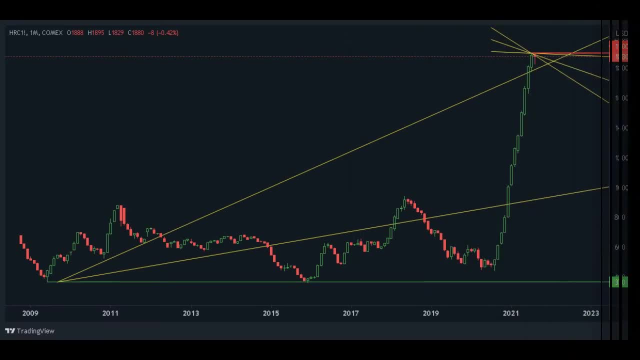 Hey guys, welcome to my analysis of flat steel futures. The global steel market is valued at nearly a trillion dollars and is expected to grow at a compounded annual growth rate of 2-3% in the coming years. The steel market is split into two types of steel products: the flat steel and the long steel. The flat steel is being the hot roll coils, cold roll coils, sheets and plates, The long steel being your rods, rounds, rails and structural elements. 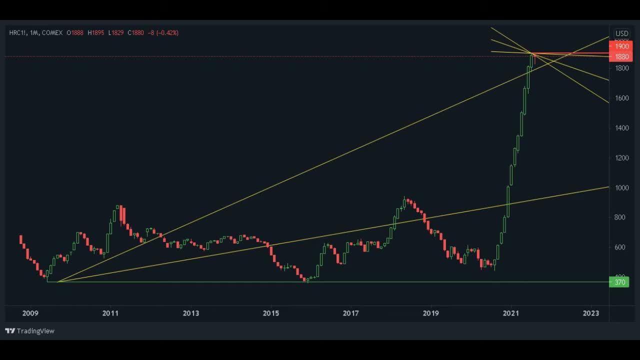 Global share of the steel market is dominated by the flat steel. Global share of the steel market is dominated by the Asia-Pacific region, which is accounting for more than 68% of the total market share, followed by Europe in second place and North America in third place. 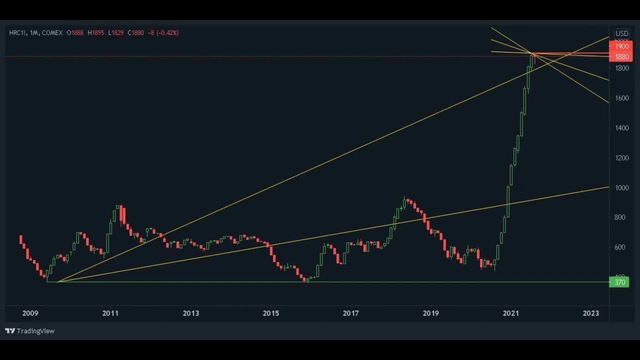 Today we are looking at the North American flat steel futures pricing. In subsequent videos I'll be covering the futures- the flat steel and long steel futures out of Shanghai, China. So, together with the North American and the Asian futures markets, we're going to do a comparison and you'll get a good idea of where the steel market is headed, what the growth is looking like, what the prices are, how the prices are shaping up, because we've already covered the raw materials which are coking- coal and iron ore in the previous videos. 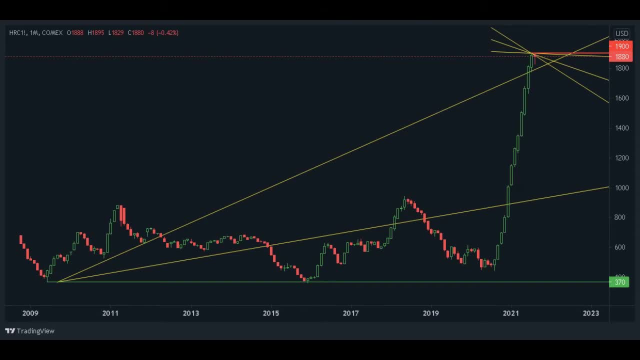 So now we're looking at the finished semi-finished steel. So we're going to look at the finished products, which are hot roll coils and rebars. What we have here is the long-term chart for the US Midwest steel hot rolled coil steel and starting from 2009: bottom of $370 to the present, where in July steel was trading at $1,900 per short ton. 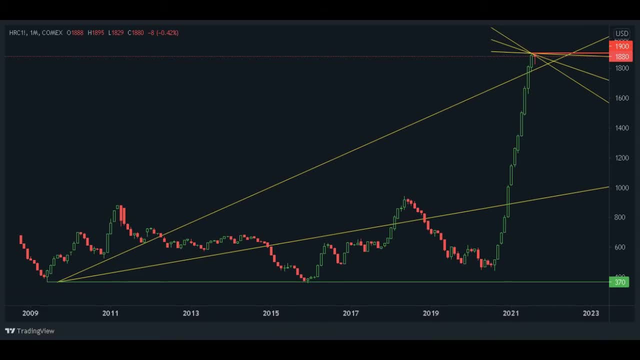 So, from the 2009 lows of $370, steel made a high of $880 in March of 2011, and then had gone sideways and finally consolidated back at the support of $370 in December of 2015,, after which it actually made a new high towards the $347.. 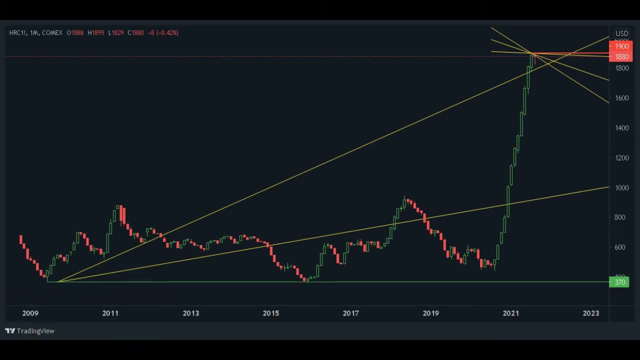 So we're going to look at the business戒 high. So we're going to look at the business戒 high At either end of percent. it was Diese emails, a polished top. That's why it's called a similar name. 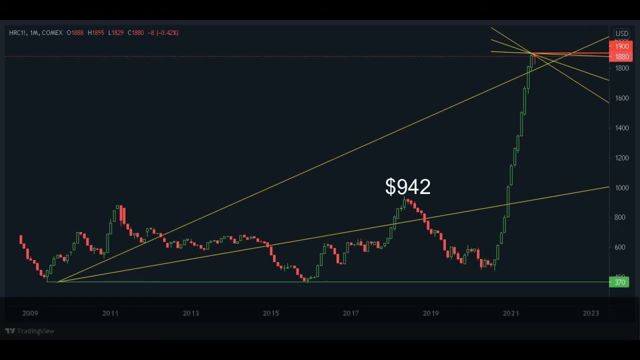 Now the policy doesn't seem to be the same, But you agree with me, So I believe that's something to be looked at. We're done, Let's go work hard together. Take a look around. OK Boy, look at that. 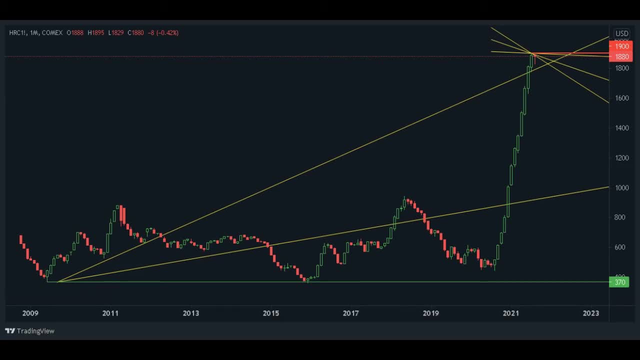 Okay, thank you all. 2018, after following which a sharp crash in steel prices towards the 522- excuse me, the 452- dollar low in april of 2020, following the covet shutdowns globally, and in 2020, until august of 2020, steel. 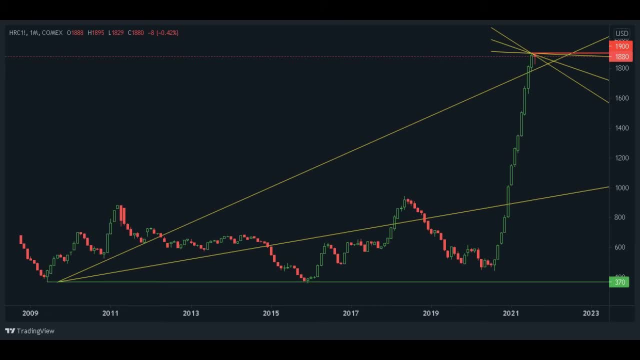 had been in a very tight range sideways market between 530 dollars and 440 dollar range, and it was only in september. only in september, end of august and beginning of september, did steel prices begin to rally again towards the 940 level and finally breaking above that and closing. 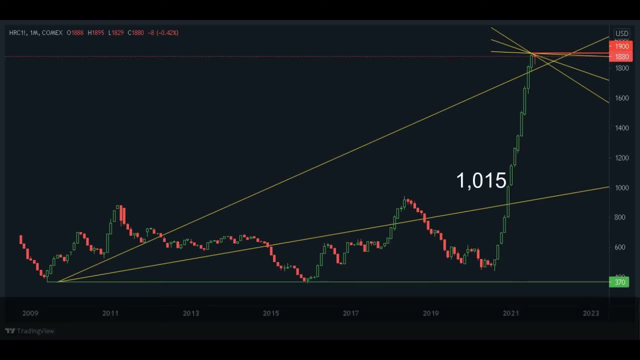 at um over a thousand dollars, a thousand fifteen, in december 2020, and it hasn't looked back since. okay, so the july, july 2020, high has been 1900 dollars, with uh hrc steel trading at eighteen hundred and eighty dollars in august. this is a gain of more than three hundred percent. 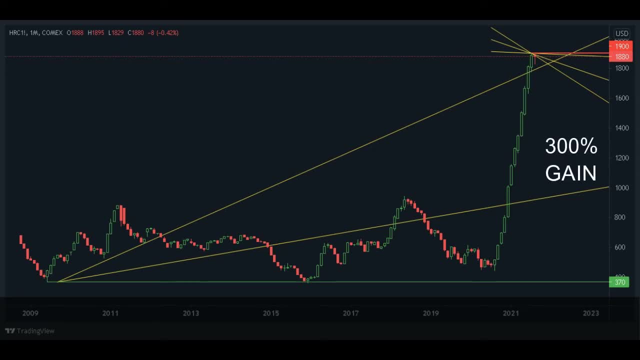 from the august bottom august 2020 till the july top of 2021. it's a huge gain. you know, 300 percent, you know in less than one year, okay so okay. a word on some technicals on the chart here. those who are not familiar with my flavor of 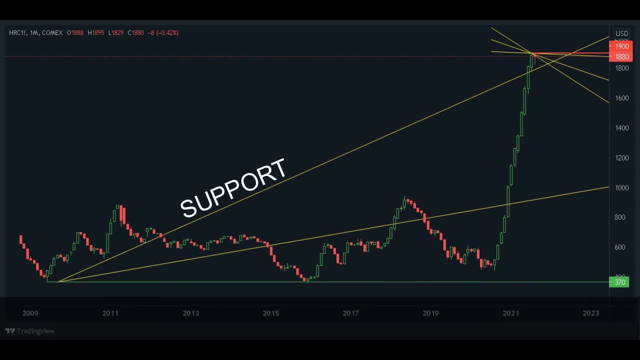 technical analysis. I want to explain what these yellow lines are on the chart. the ones that are emanating from the bottom up, the bottom of three hundred seventy dollars going up- okay, they are supports in prices and time, while the ones that are emanating from the top, from the from the top made in July last. 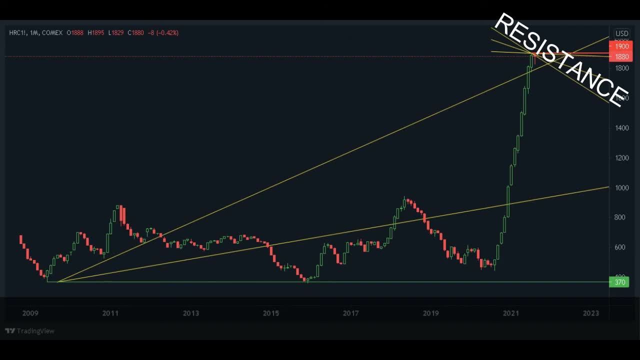 month of nineteen hundred dollars going down. these three lines are your resistance levels in price and time. okay, so now we know what steel has done in the past, since 2009. what interests us is what steel will do do in the future. what? what the prices, how the prices are shaping up in for the 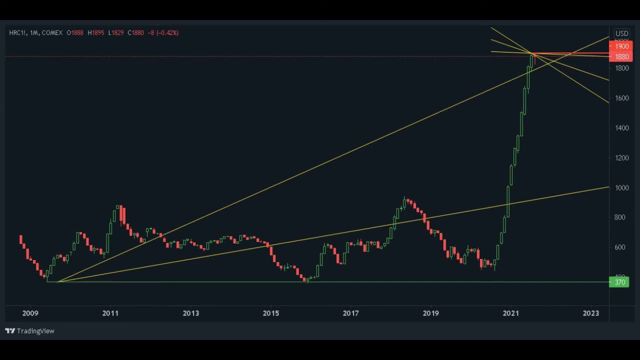 rest of August, going into September and the rest of the year. as you can see on the chart, the seventeen hundred and ninety dollar support level in August is a very, very important long-term support on the trend line emanating from 2009 September. okay, so we have nearly tested that. we made a low of 1829 in August and 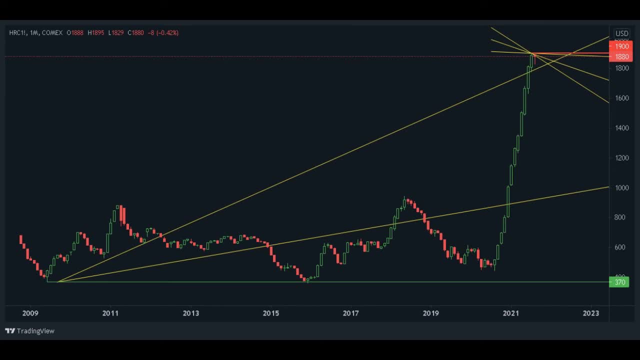 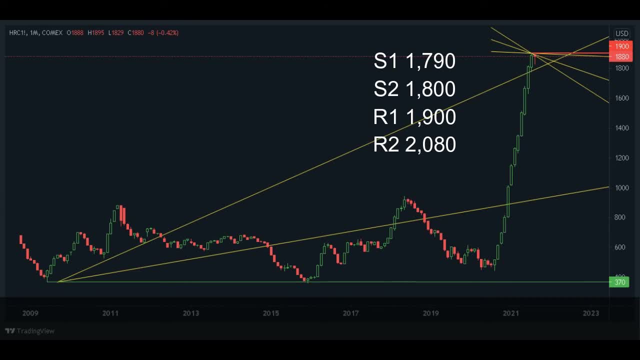 okay. so, depending on where the prices end up the month end. if it is above 1900: okay. so, depending on where the prices end up the month end. if it is above 1900: okay. so, depending on where the prices end up the month end. if it is above 1900, which is its first resistance, then the 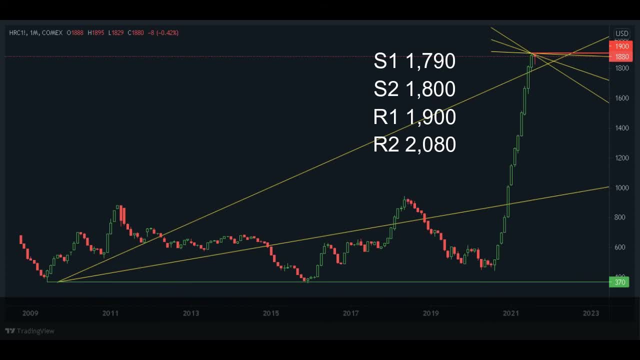 which is its first resistance, then the, which is its first resistance, then the bullish run is is to continue towards bullish run. is is to continue towards bullish run. is is to continue towards the 2000- 2000 plus 2080 dollar level in the 2000- 2000 plus 2080 dollar level in. 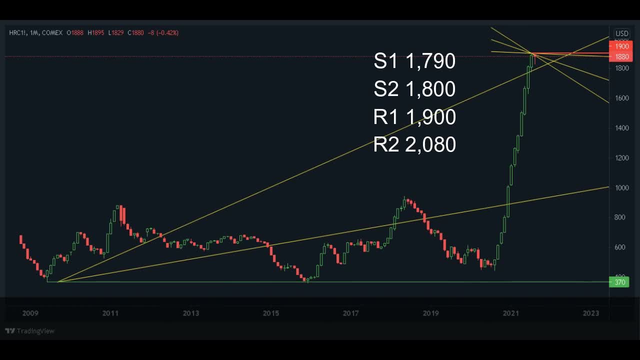 the 2000, 2000 plus 2080 dollar level in September, okay, let me repeat that. if September, okay, let me repeat that. if September, okay, let me repeat that. if August closes above 1900, then September. August closes above 1900, then September. 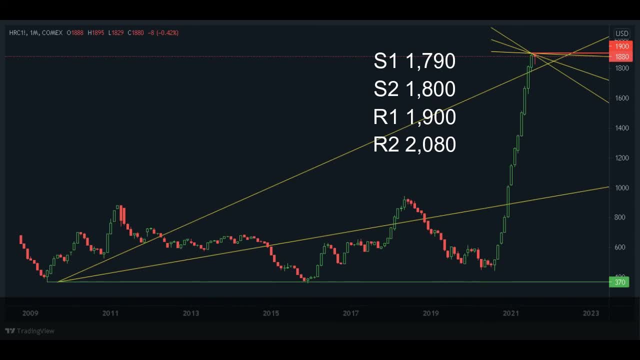 expected to be towards the two thousand eighty dollar level, else we could be retesting eighteen hundred, eighteen hundred again. the support level, the long-term support level back in September, will be retesting eighteen hundred. if August closes below nineteen hundred, okay, and if the eighteen hundred level holds, we can expect that October could be bullish, that steel prices would. 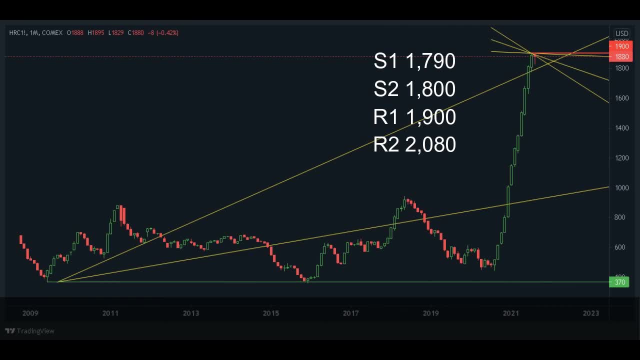 try again to break above the nineteen hundred resistance made in July, the high made in July towards the, and if it's successful in breaking that and we can expect November and December prices to be over two thousand towards the two thousand eighty dollar resistance for 2021. okay, guys, so I just shared an 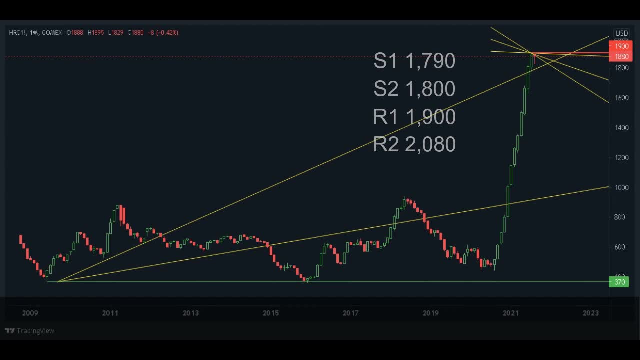 important level for you for this year. for the rest of the year, two thousand and eighty dollars for HRC steel futures out of the US Midwest is gonna be the high and the resistance to break in 2022. okay, so if eighteen hundred dollar level holds, then steel 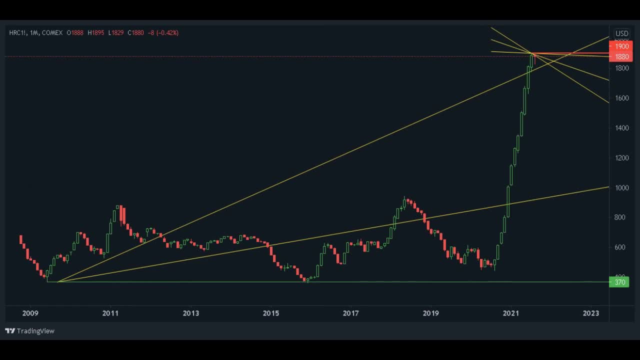 futures still have a future above nineteen hundred. else we're gonna see some corrections and which we'll cover as and when it happens. before that support level breaks. I'll come back to you with more information and and the path forward. but as of right now, there's no reason to believe that the eighteen 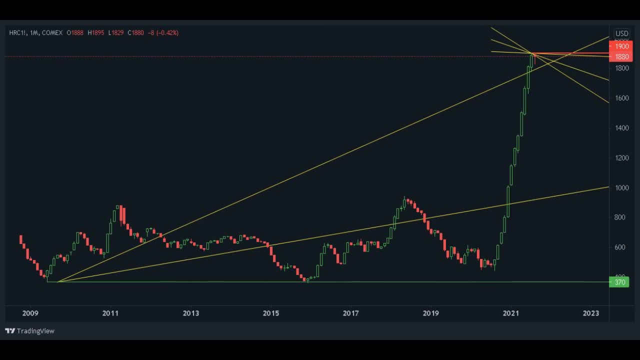 hundred dollar support level will break anytime soon and we will resume our uptrend again in October and topping out at twenty eighty by the end of 2021, by December twenty twenty one. so thank you, guys. that's. that's all I have for you for HRC futures analysis. if you have any questions, as always, put them down in. 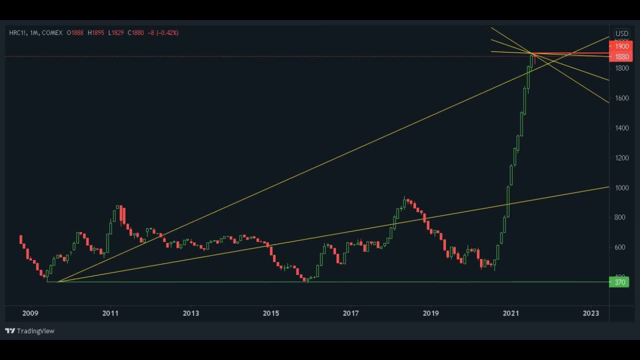 the comment section or you can contact me directly and I will get back to you and thank you for listening and do look forward to the Shanghai steel market futures analysis. this is a. we're looking at the longs and flats there, the rebar futures and the hot roll coil futures out of Shanghai, China next. take care and bye, bye you.